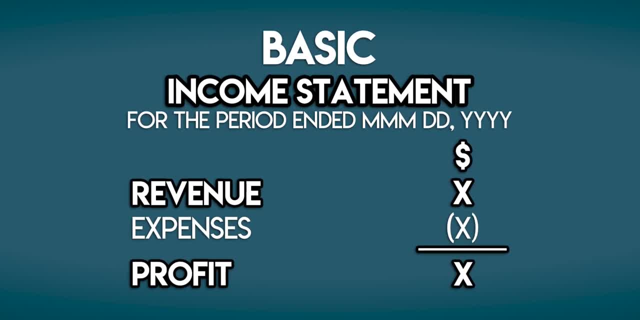 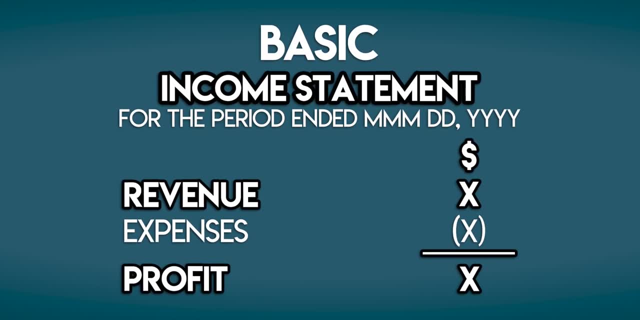 and expenses incurred over a period of time. Profit is the difference. It's the financial gain generated when revenues are bigger than expenses. Alright, so what does profit mean? Why is it important? Why are you paying a lot of money? Why are you placing your money on your business? 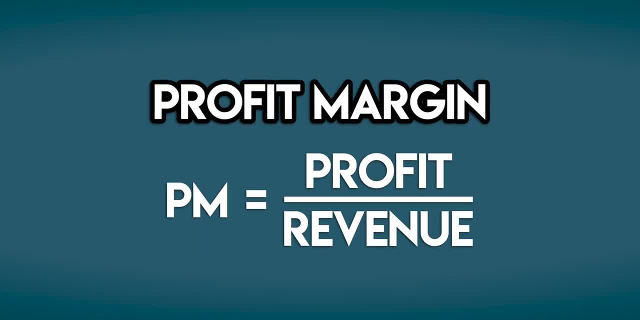 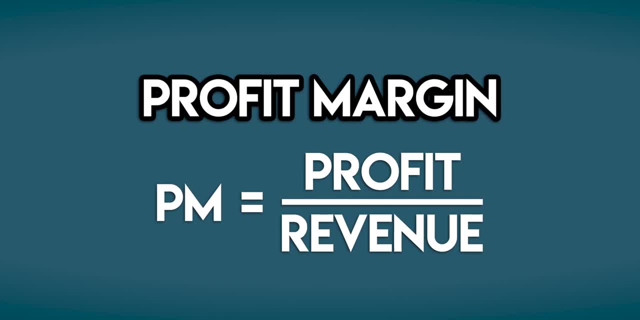 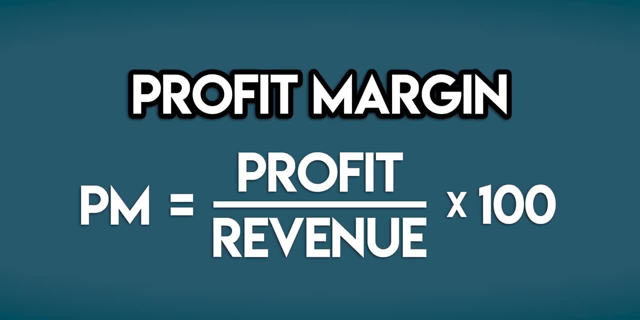 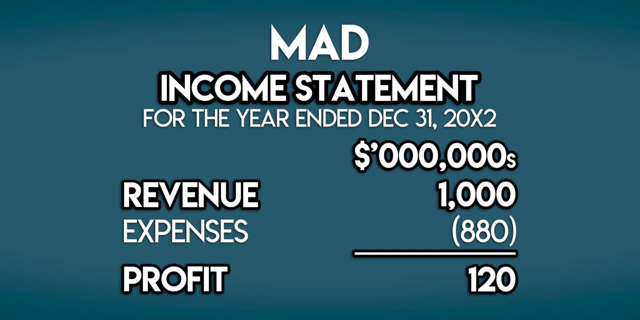 shows us how much profit a business generates for each dollar of revenue earned, or, when we times it by 100, what percentage of revenue is able to convert into profit. for example, here's the income statement for a business called MAD. they're a tech company that makes processors and graphics cards out of. 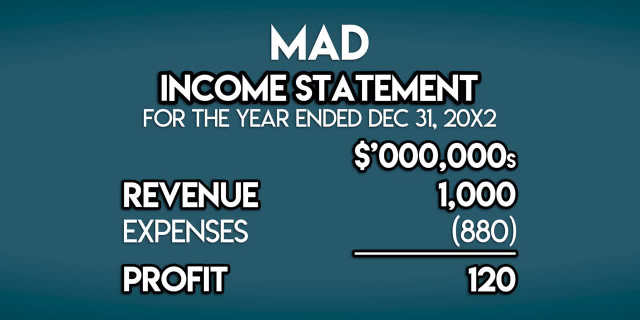 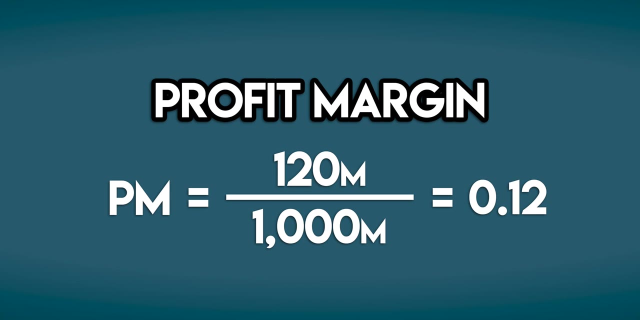 California. last year, MAD earned 1 billion dollars in revenue and they incurred 880 million dollars in expenses. the difference of 120 million dollars is their profit, which is the financial gain to their business. MAD's profit margin is 120 million dollars divided by 1 billion dollars. that's 12 cents of profit. 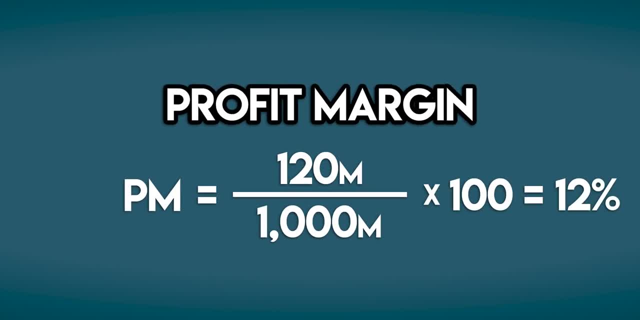 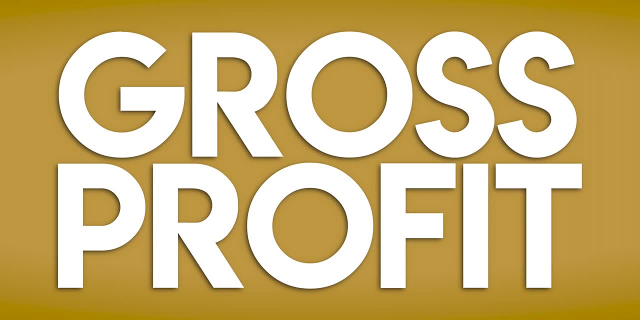 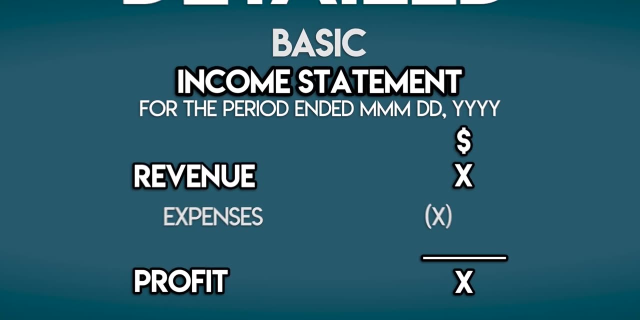 generated on every dollar of revenue earned a 12% profit margin. if we multiply by a hundred, now, how does gross profit fit into all of this? let's jump back to the income statement. this one's very compressed. in reality, businesses split out their expenses into a few. 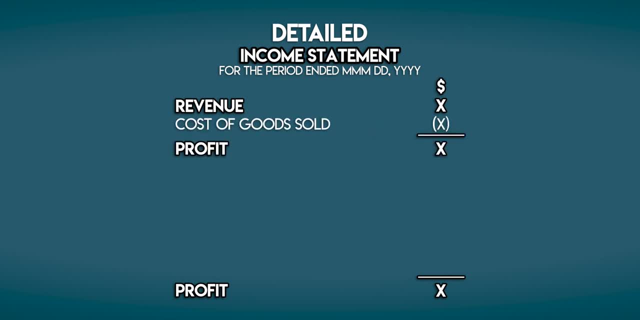 different buckets. first we take away the direct cost of sales, then all the indirect operating costs like research and development, selling general and financing, savings, depreciation and amortisation and finally we subtract interest and tax expenses. as you can see, the income statement shows three different types of profit. the big one at the top is called gross profit. the 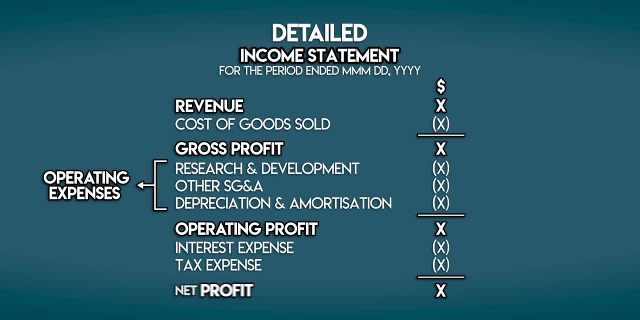 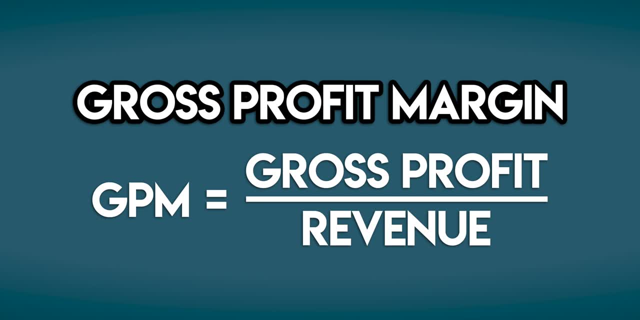 middle one is operating profit and the smallest one at the bottom is net profit, the bottom line. so what is gross profit margin? at the start we said the gross profit margin is a business's gross profit margin and the sum of the first ten plus interest payments is therefore basically being mostly zero. bank represents. 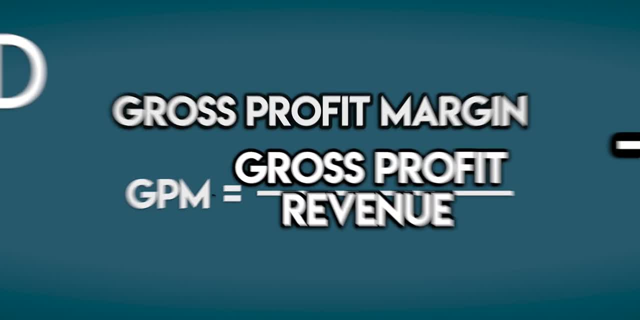 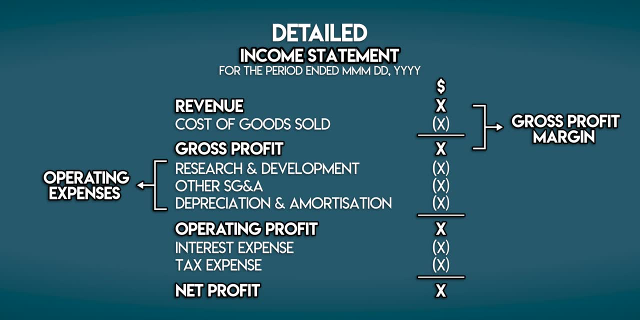 divided by its revenue, It measures how much big profit they're able to generate from each dollar of revenue they earn. Gross profit margin only factors in a business's direct cost of sales. It totally ignores all of the indirect operating expenses, interest and tax that we can see. 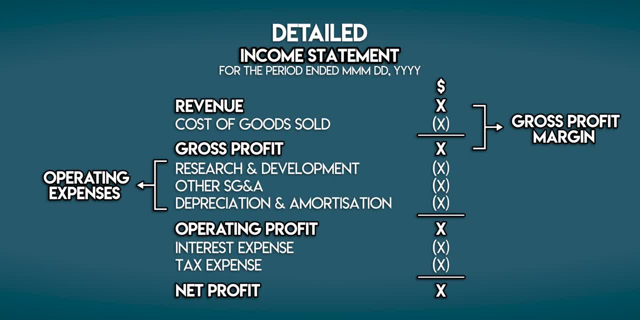 further down the income statement. We use different ratios to measure those which I'll explain in my next videos, so remember to click subscribe if you'd like to see them. I've also put together a new cheat sheet which shows all the different profitability ratios, If you'd like to. 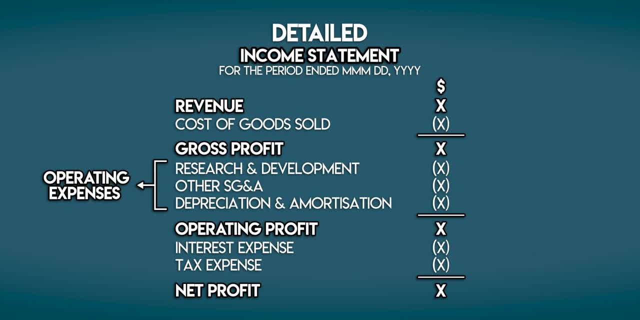 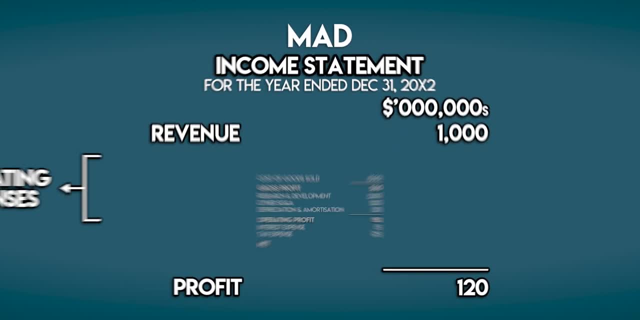 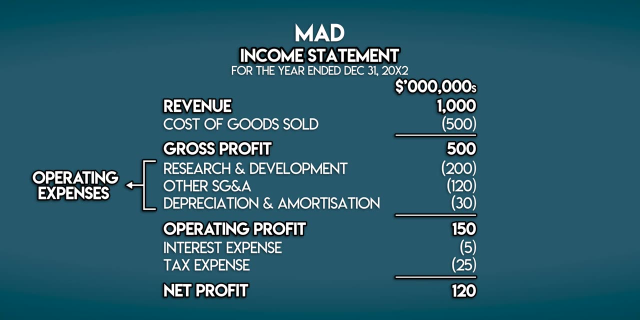 support this channel, then you can buy it on my website. The link's in the description. Example time: What was MAD's gross profit last year? If we expand out their income statement, we can see that they earned revenue of one billion dollars and they incurred 500 million dollars in cost of. 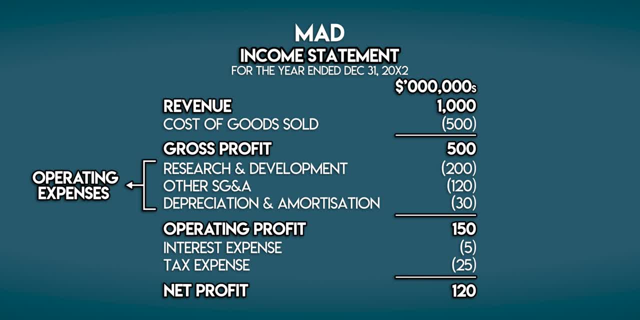 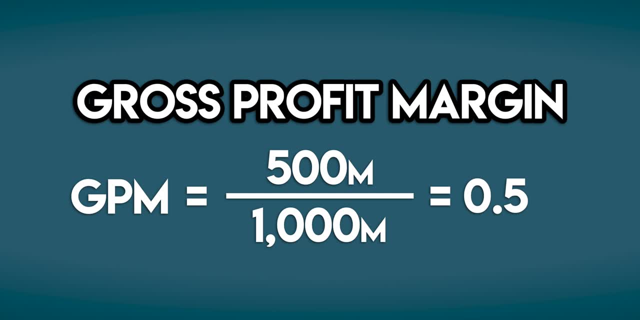 goods. That left them with a gain in gross profit of 500 million dollars. So their gross profit margin is 500 million dollars in gross profit divided by one billion dollars in revenue. That's 50 cents of gross profit generated on each dollar earned, or 50% if we multiply by 100.. But how should we? 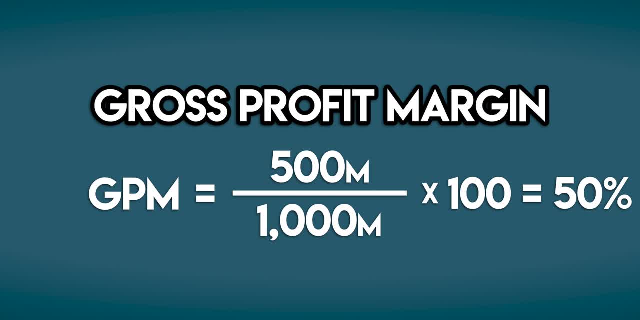 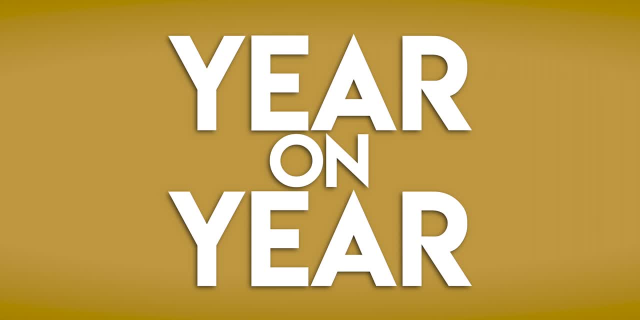 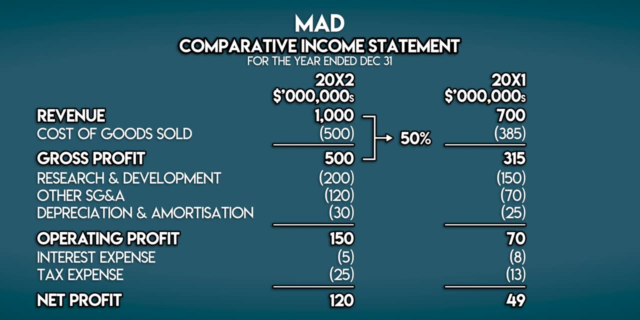 interpret this Is 50% good or bad. It's hard to say, so let's make some comparisons. First, what's the year-on-year movement in gross profit margin? Let's compare MAD's current and prior year income statements. We can see that they had a gross profit of 315 million dollars in the previous. 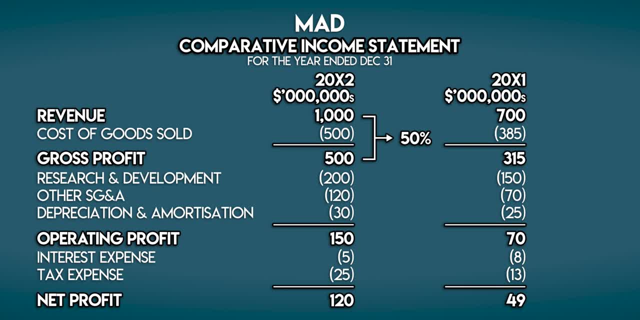 year. When we divide that by their revenue of 700 million dollars, that's a gross profit margin of 45%. So MAD managed to raise their gross profit margin by 5% year-on-year. That's good news, because bigger is better. They managed to generate five extra cents of gross profit on each dollar they earned. 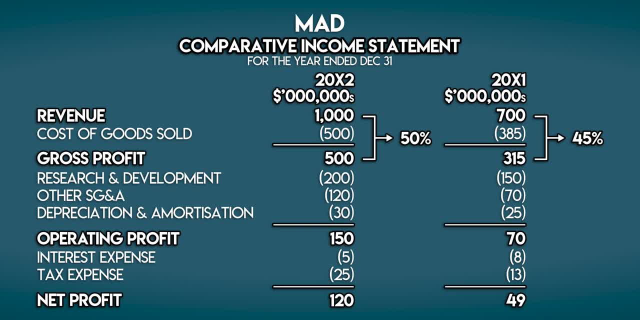 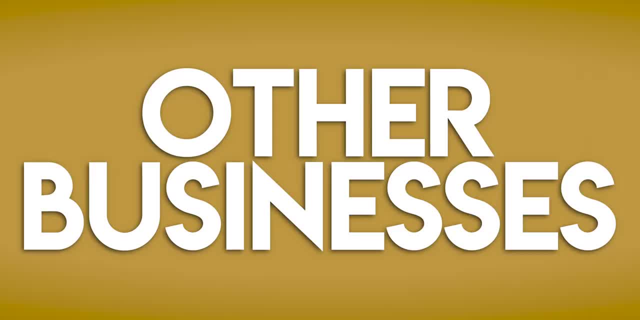 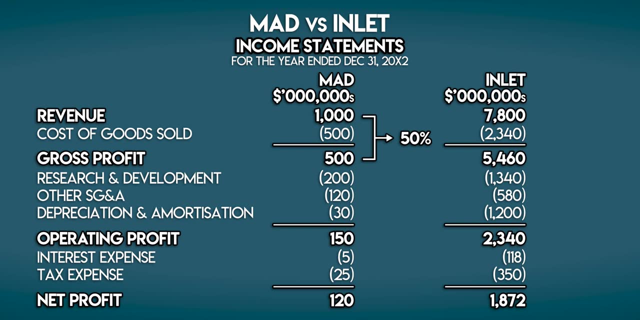 They also managed to increase their revenue from 700 million dollars to one billion dollars. Things are looking promising, But how does their gross profit margin compare against their competitors? Here are the current year income statements for MAD and Inlet, Both of these businesses.